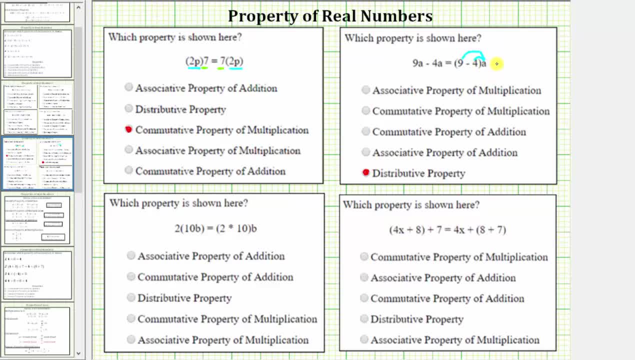 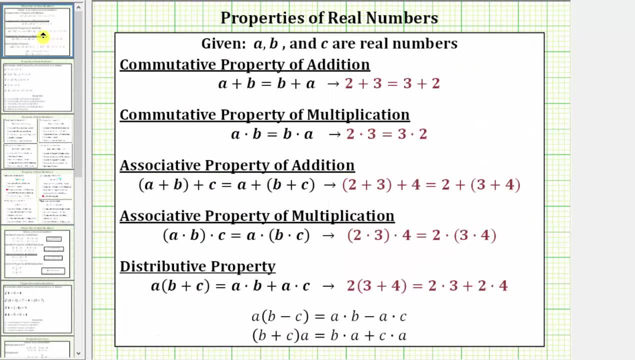 And for this particular example, we distributed from the right, and it's also possible and more common to distribute from the left. Looking at our notes, the distributive property is normally expressed as a times. the quantity b plus c equals a times b plus a times c. 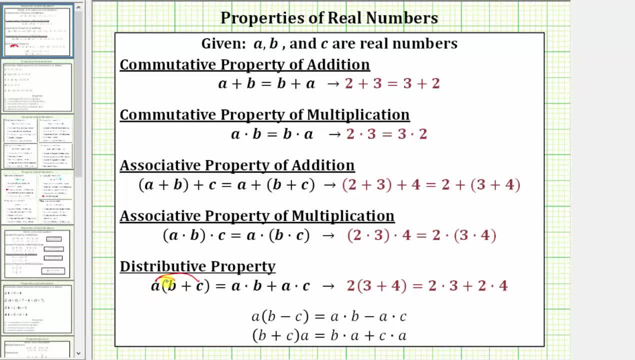 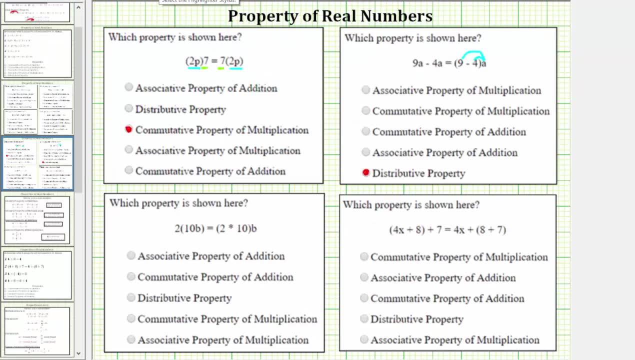 where we distributed the a from the left. But our example fits this form here, where we have the quantity b plus c times a equals b times a plus c times a. Both demonstrate the distributive property. Next we have 2 times the quantity 10b. 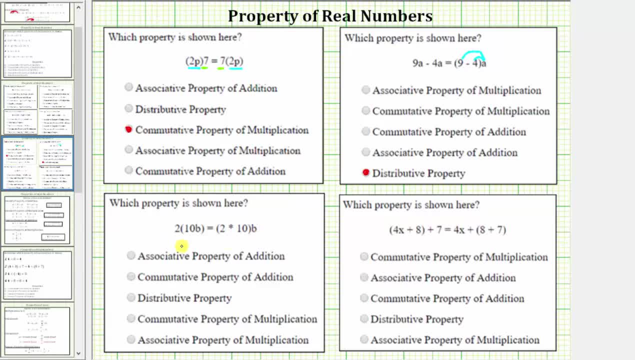 Notice: on both sides of the equation we have a product, but the grouping of the factors has changed. Notice: on the left we have grouping symbols or parentheses around 10 times b or 10b. On the right, we have grouping symbols or parentheses around the 2 times 10.. 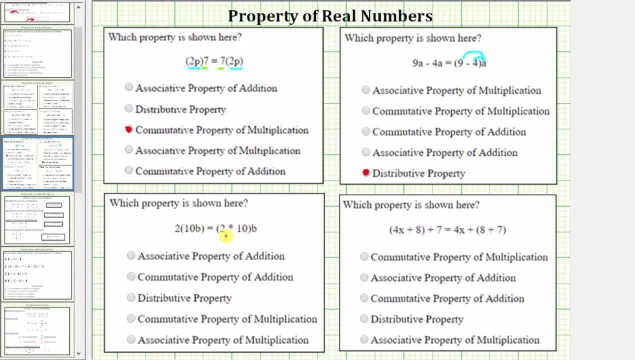 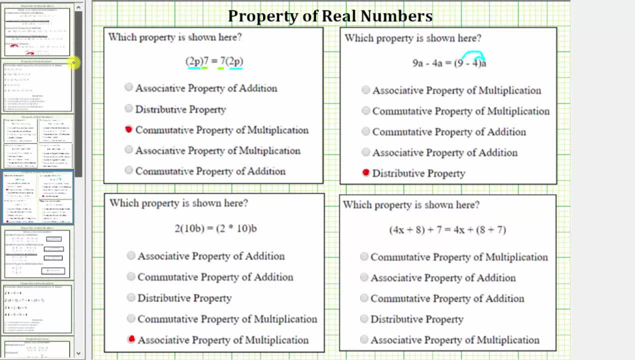 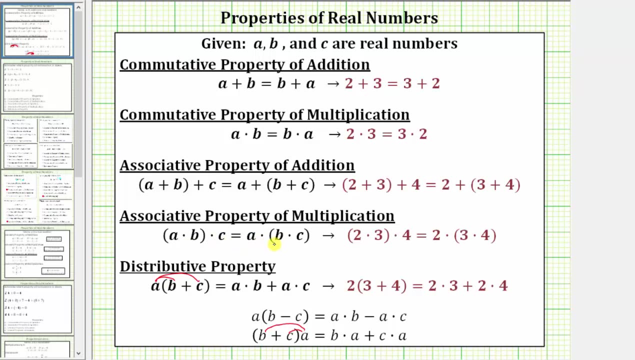 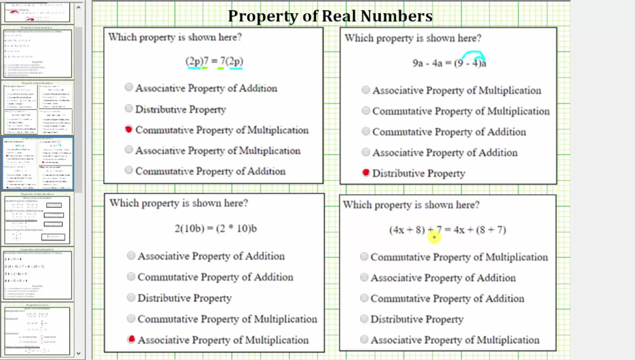 Because the grouping of the product has changed. this is an example of the associative property of multiplication. This is normally expressed as: the quantity a times b times c equals a times the quantity b times c. For the last example, we have the quantity 4x plus 8 plus 7 equals 4x plus the quantity. 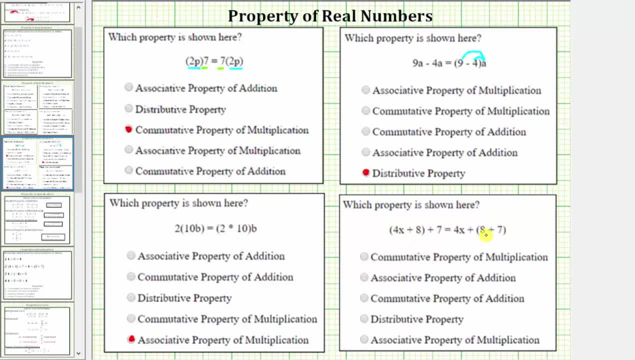 8 plus 7.. Notice: on both sides of the equation we have a sum and the order of the terms is the same, but the grouping of the terms in the sum has changed. Notice: on the left we have grouping symbols or parentheses around the sum 4x plus 8.. 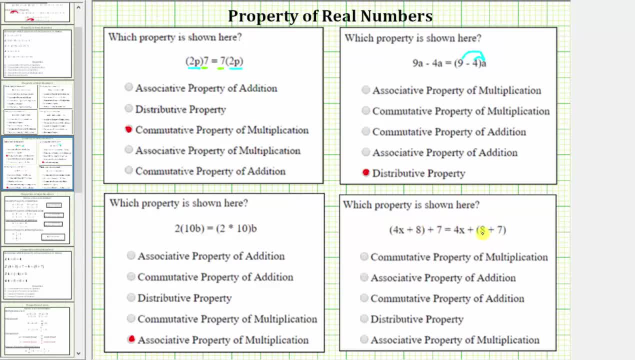 On the right we have parentheses or grouping symbols around the sum 8 plus 7.. So, because the grouping of the sum has changed, this is an example of the associative property of addition. More formally, this property is often expressed as the quantity a plus b plus c equals a plus.